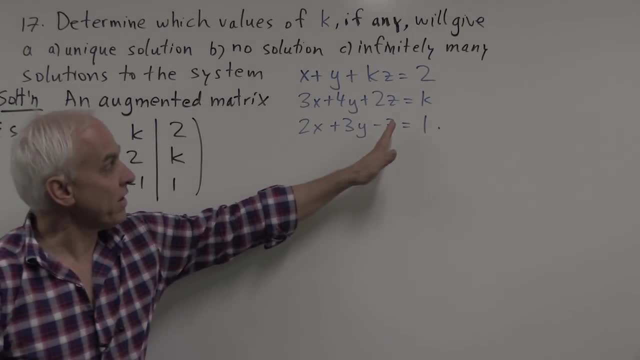 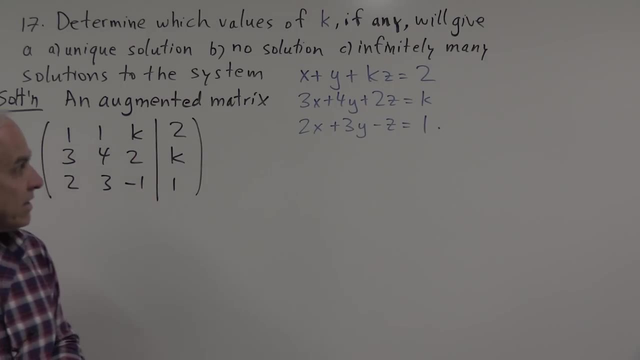 Alright, so we've just written down the coefficients of the x, y and z on the left-hand side, that part of the matrix, the coefficient part of the matrix, and the right-hand side, 2k1 on the right-hand side there. 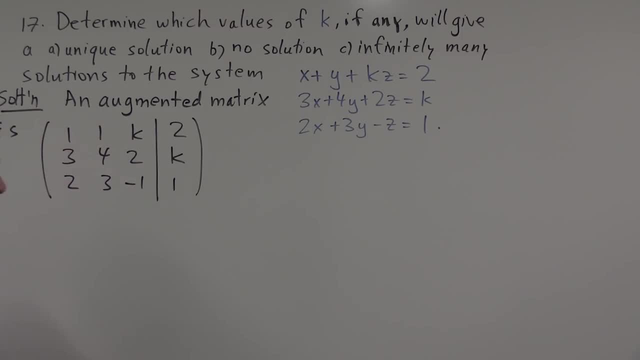 Alright, now we're going to row reduce, just as we usually do, try to ignore the fact that there's a k instead of a number. So we'll start with this entry here as a pivot entry and we're going to use it to eliminate the entries in the column below it. 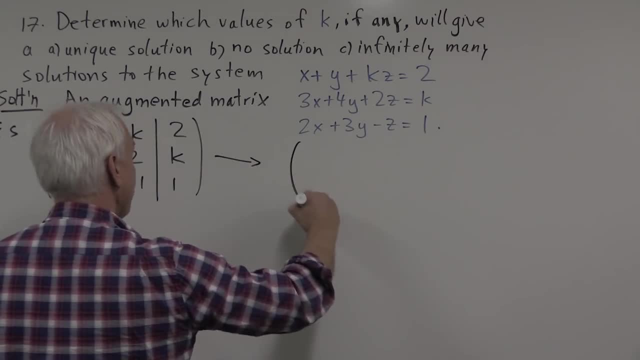 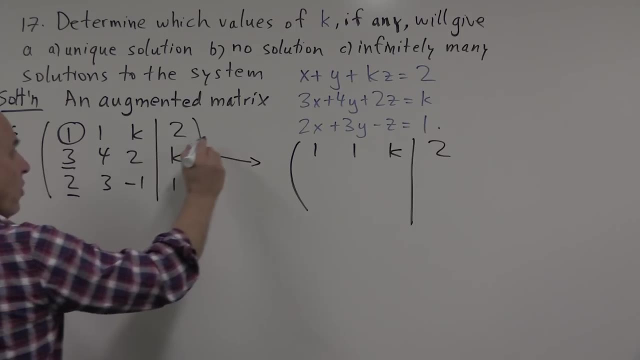 Alright, so what happens? So we're going to get this: will still be 1,, 1,, k, 2, that first row doesn't change, And we're going to take row 2, and our new row 2 will be row 2, minus 3,, 2, and k. 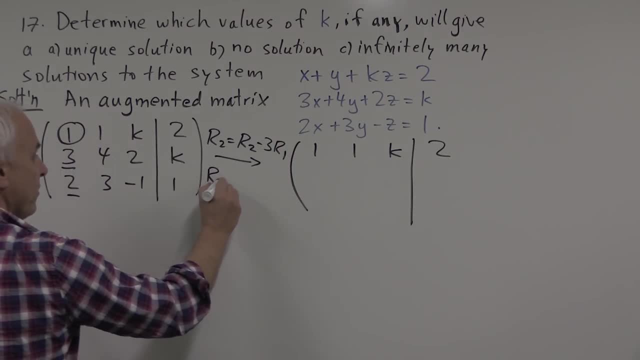 3 times row 1.. And our new row 3 will be the old row 3, minus 2 times row 1.. Alright, so we take row 2, and we subtract 3 times row 1.. What do we get? 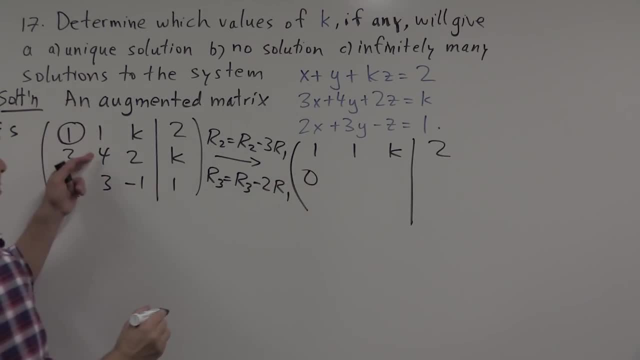 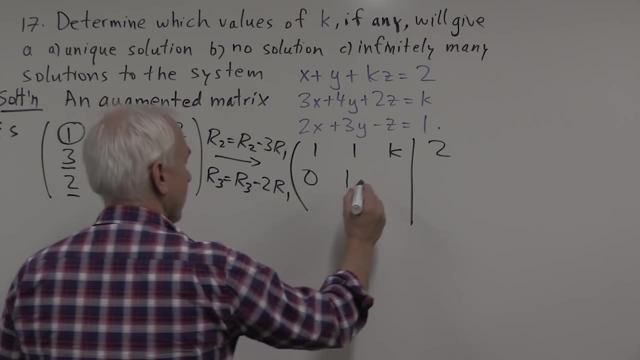 3 minus 3 times 1 is 0.. 4 minus 3 times 1 happens to be 1.. And 2 minus 3k is well, it's just 2 minus 3k. that's all we can say. 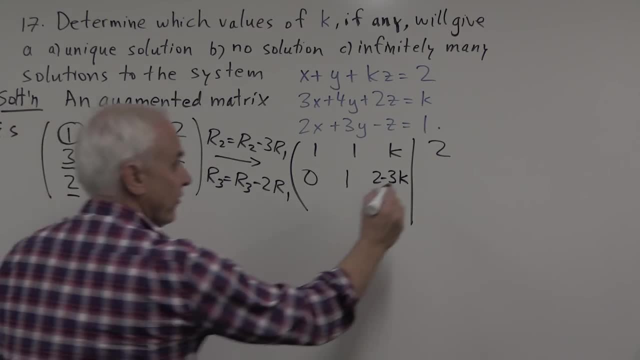 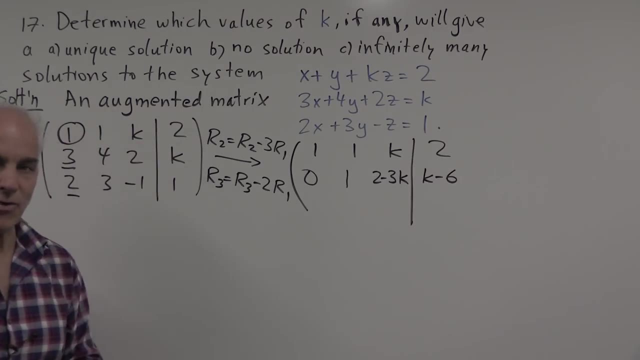 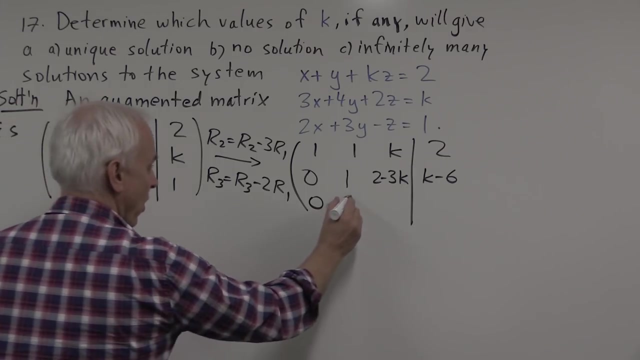 And k minus 3 times 2 is k minus 6.. For the third row we have to take it and subtract 2 times row 1.. 2 minus 2 times 1 is 0.. 3 minus 2 times 1 is 1.. 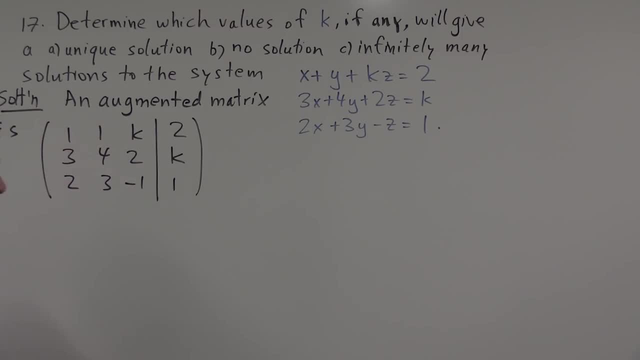 Alright, now we're going to row reduce, just as we usually do, try to ignore the fact that there's a k instead of a number. So we'll start with this entry here as a pivot entry and we're going to use it to eliminate the entries in the column below it. 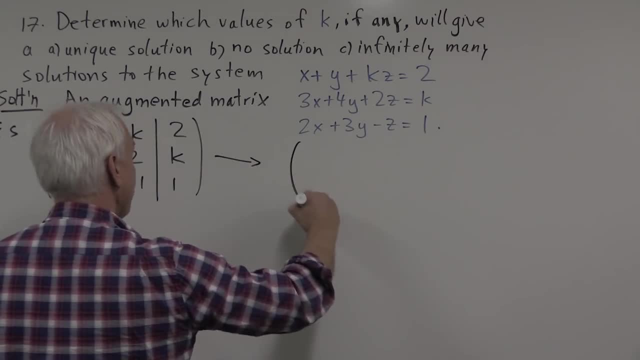 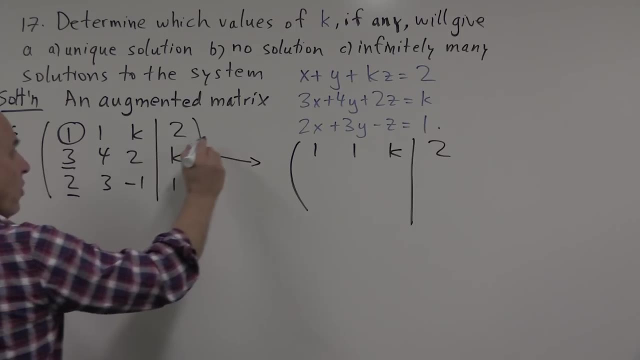 Alright, so what happens? So we're going to get this: will still be 1,, 1,, k, 2, that first row doesn't change, And we're going to take row 2, and our new row 2 will be row 2, minus 3,, 2, and k. 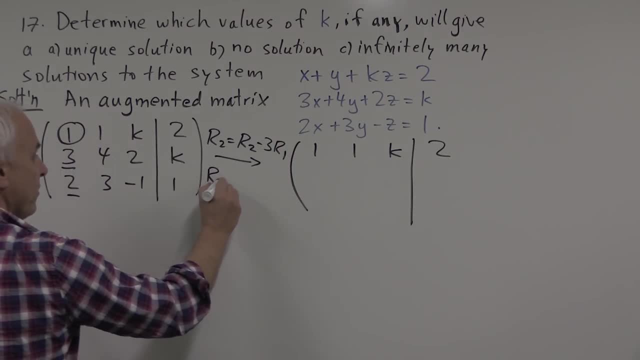 3 times row 1.. And our new row 3 will be the old row 3, minus 2 times row 1.. Alright, so we take row 2, and we subtract 3 times row 1.. What do we get? 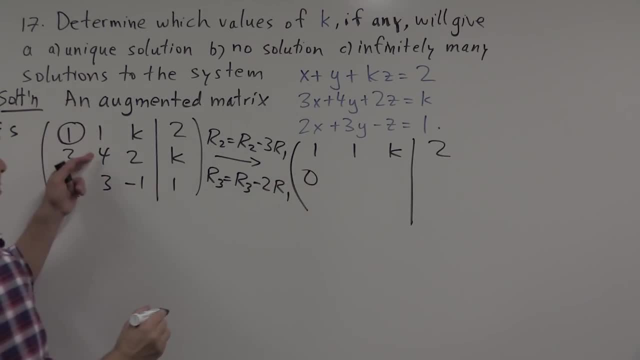 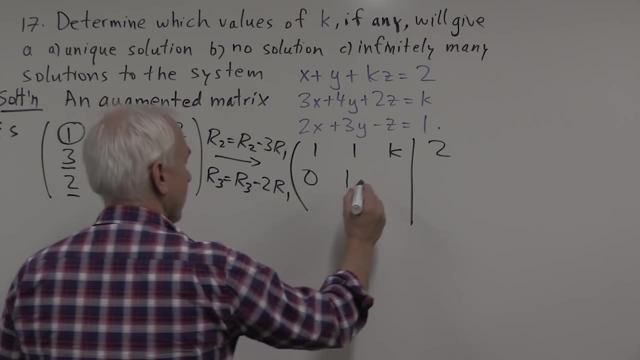 3 minus 3 times 1 is 0.. 4 minus 3 times 1 happens to be 1.. And 2 minus 3k is well, it's just 2 minus 3k. that's all we can say. 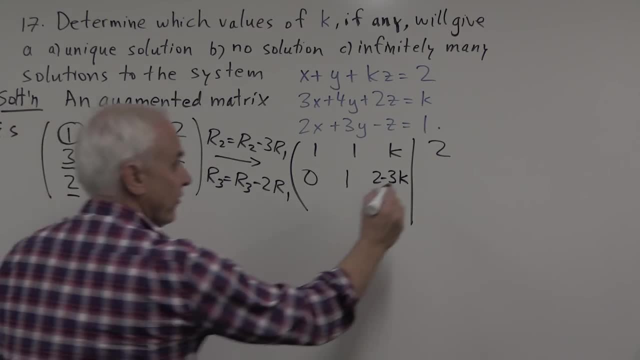 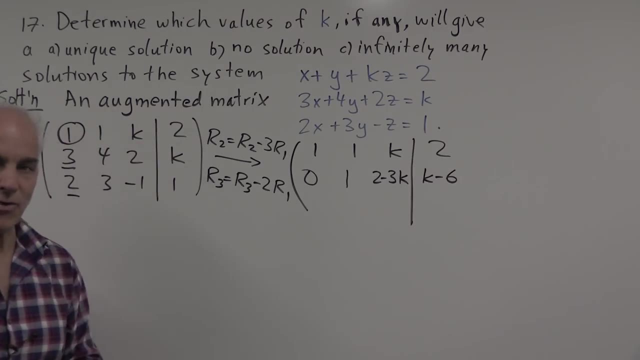 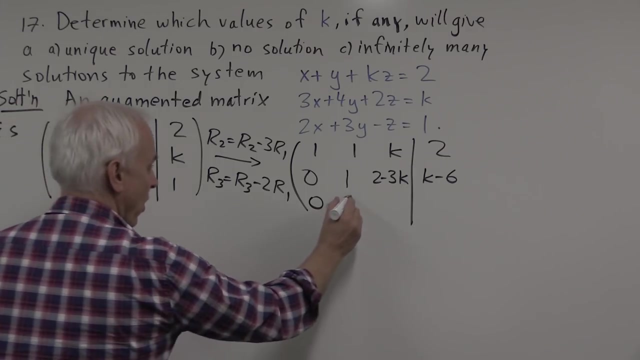 And k minus 3 times 2 is k minus 6.. For the third row we have to take it and subtract 2 times row 1.. 2 minus 2 times 1 is 0.. 3 minus 2 times 1 is 1.. 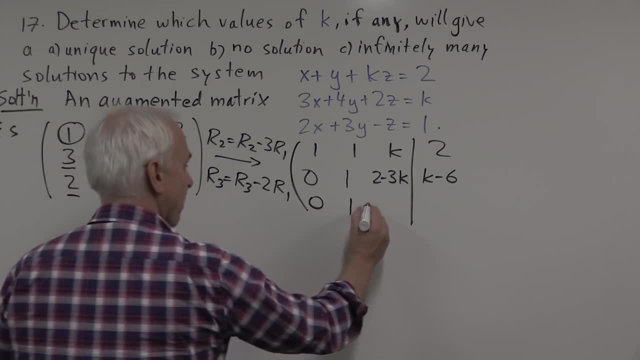 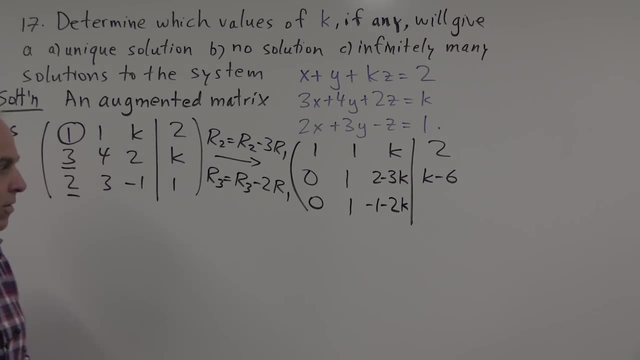 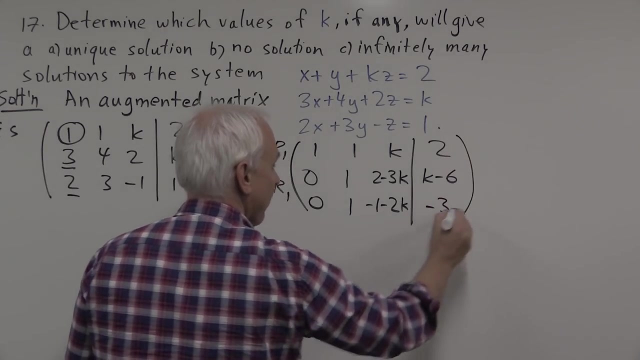 And minus 1 minus 2 times this will be minus 1 minus 2k. We'll just treat the k as a variable whose value we don't know. And finally, 1 minus 2 times 2 will be minus 3.. 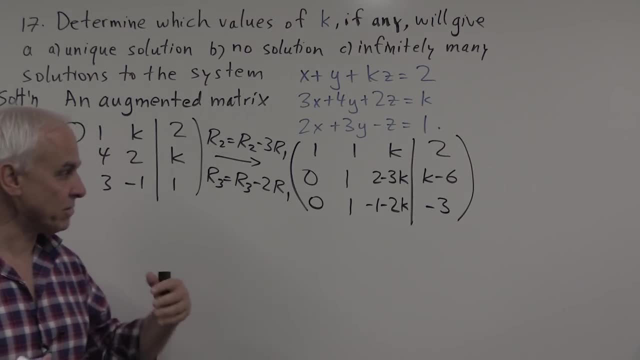 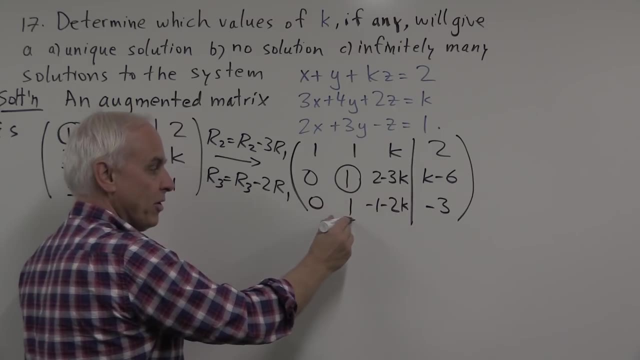 Alright, it's a little bit complicated now because there's this k involved instead of numbers, but we're still going to proceed with our row reduction. see what it gets us. So in our next step, we take this 1 as our pivot entry and we're going to eliminate the 1 below it. 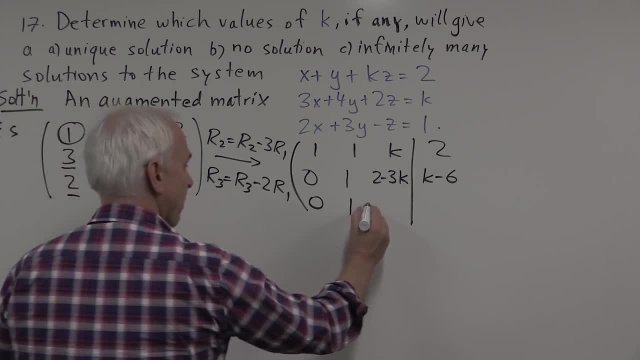 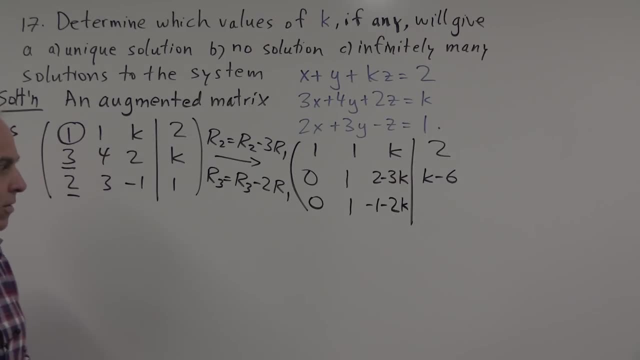 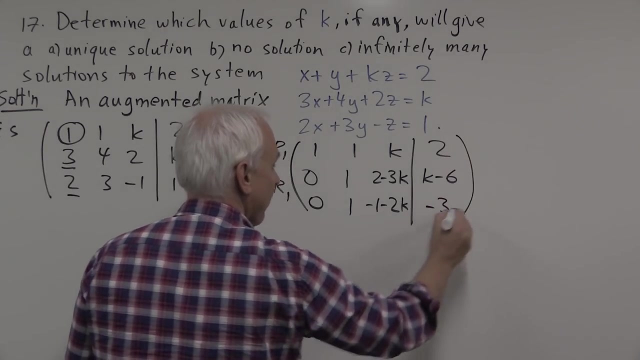 And minus 1 minus 2 times, this will be minus 1 minus 2k. We'll just treat the k as a variable whose value we don't know. 1 minus 2 times 2 will be minus 3.. Alright, it's a little bit complicated now, because there's this k involved instead of numbers. 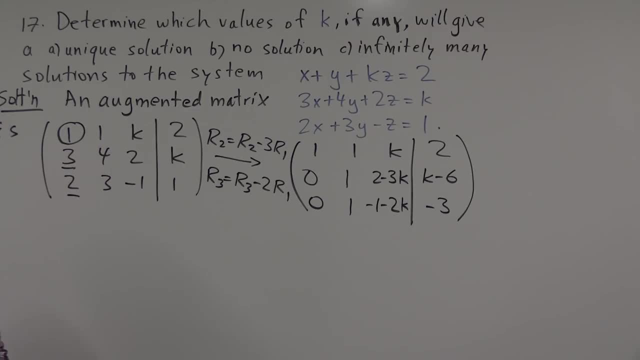 but we're still going to proceed with our row reduction. see what it gets us. So in our next step, we take this 1 as our pivot entry and we're going to eliminate the 1 below it. Alright, so going over here, we're going to have 1,, 1,. I'll leave a little bit more room here now. 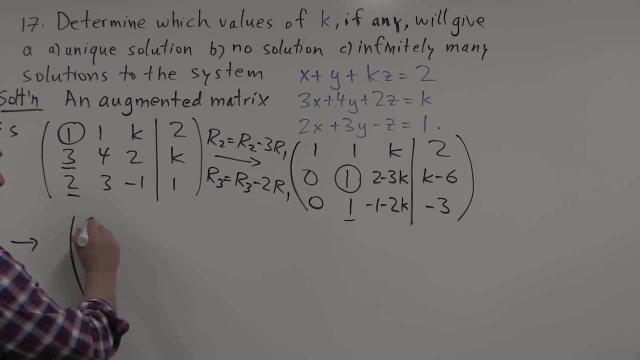 Alright. so going over here we're going to have 1,, 1,. I'll leave a little bit more room here now because it might get a little bit more complicated. It's complicated algebraically And 0,, 1, and here we have 2 minus 3k and k minus 6.. 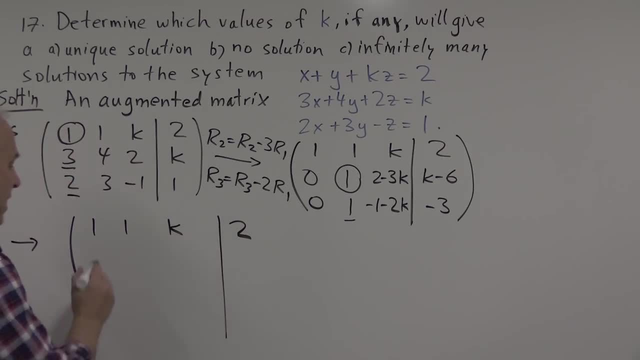 because it might get a little bit more complicated algebraically- And 0,, 1, and here we have 2 minus 3k and k minus 6.. Alright, so we're going to take row 3 is going to be row 3 minus row 2.. 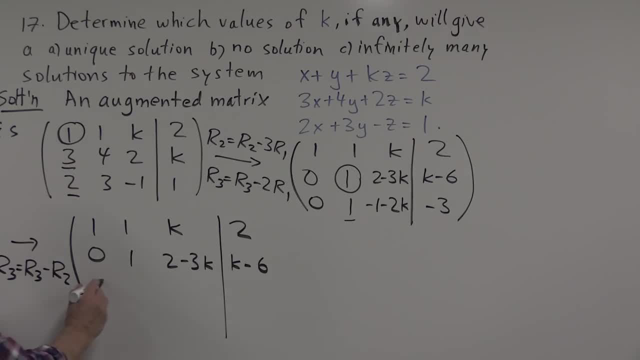 Take this row and subtract row 2 from it. That'll give us 0.. 1 minus 1 is 0.. And then over here we have minus 1 minus 2k, minus 2 minus 3k, So this entry minus this. 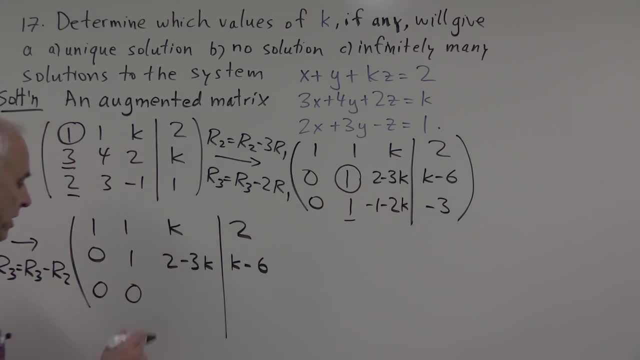 Well, I think we can do that in our heads: Minus 1 minus 2 will be minus 3.. And minus 2k minus minus 3k will be minus 2k plus 3k, for a total of plus k. 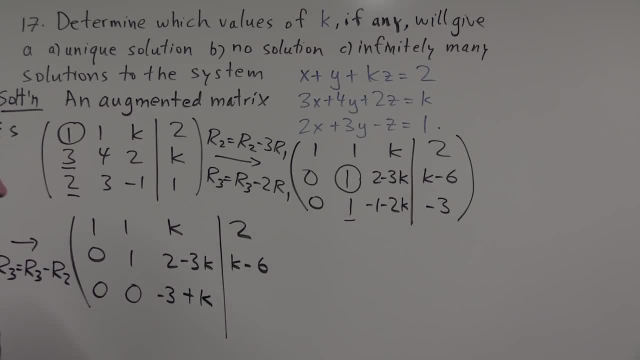 And then over here on this side we'll have minus 3, and then we have to subtract k minus 6.. So minus 3 minus k minus 6.. That's minus 3 plus 6, so it'll be plus 3 and minus k. 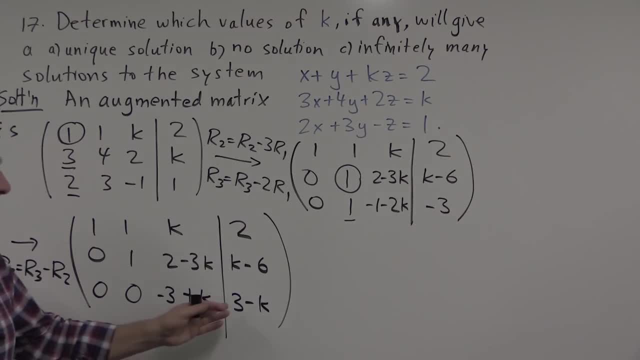 This thing minus this, will be 3 minus k. Okay, and now we are in a position to try to figure out whether or not this thing has solutions and, if so, how many solutions it has, And it will depend on the values of k. 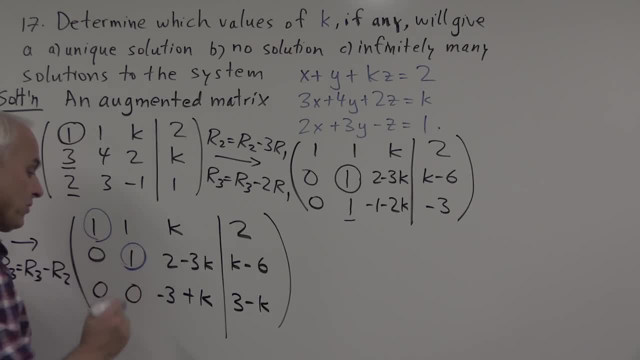 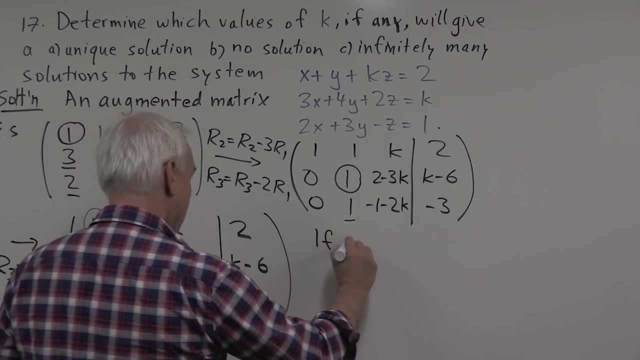 So here we have a leading entry, and here we have a leading entry And this is possibly a leading entry. It will be a leading entry if it is non-zero, So we can say that if minus 3 plus k does not equal 0,. 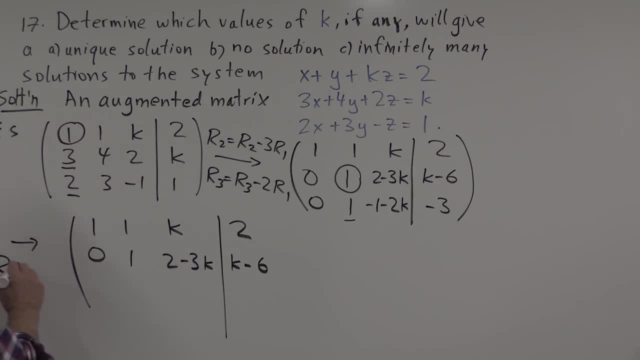 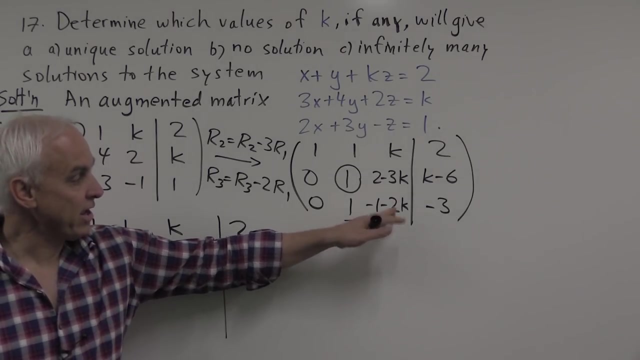 Alright, so we're going to take row 3 is going to be row 3 minus row 2.. Take this row and subtract row 2 from it. That'll give us 0.. 1 minus 1 is 0.. And then over here we have: minus 1 minus 2k. minus 2 minus 3k. 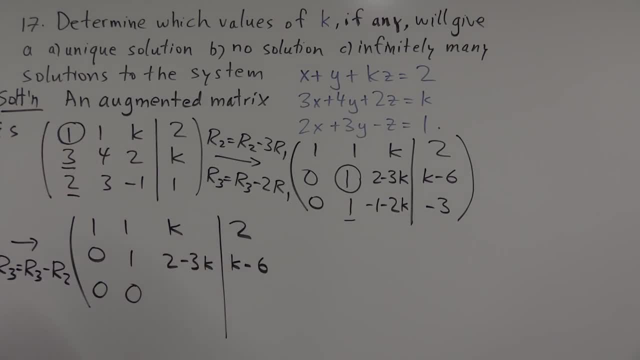 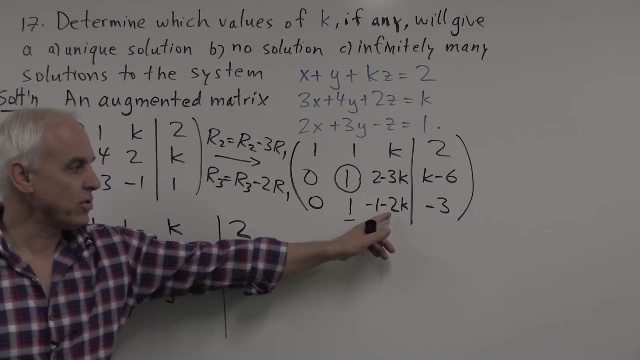 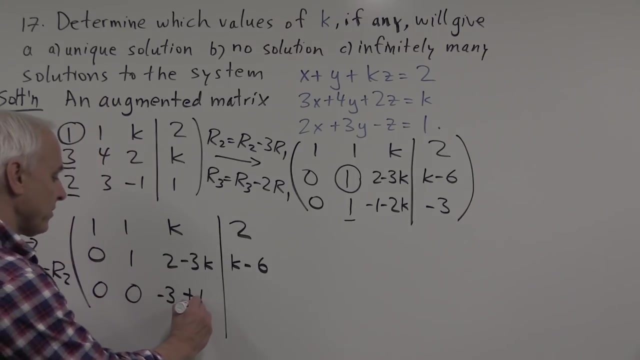 Alright. So this entry minus this. Well, I think we can do that in our heads: Minus 1 minus 2 will be minus 3.. And minus 2k minus minus 3k will be minus 2k plus 3k, for a total of plus k. 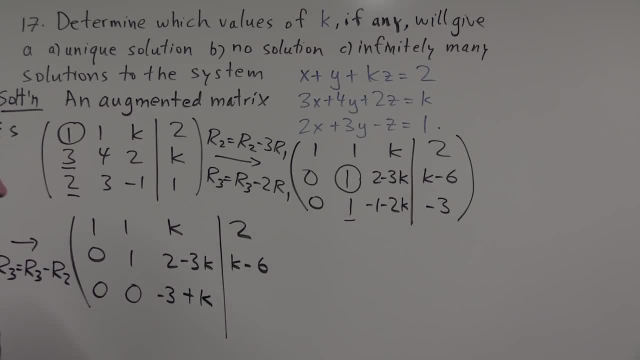 And then over here on this side we'll have minus 3, and then we have to subtract k minus 6.. So minus 3 minus k minus 6.. That's minus 3 plus 6.. So it'll be plus 3 and minus k. 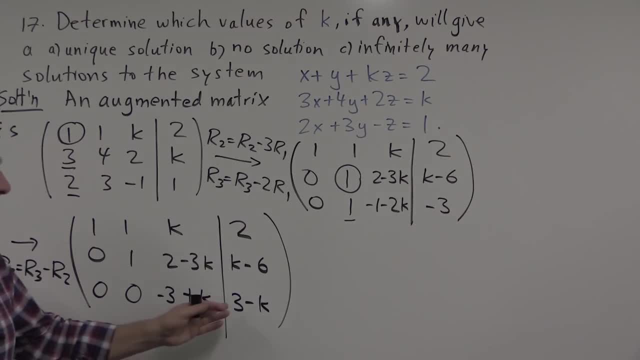 This thing minus this, will be 3 minus k. Okay, And now we are in a position to try to figure out whether or not this thing has solutions And, if so, how many solutions it has, And it will depend on the values of k. 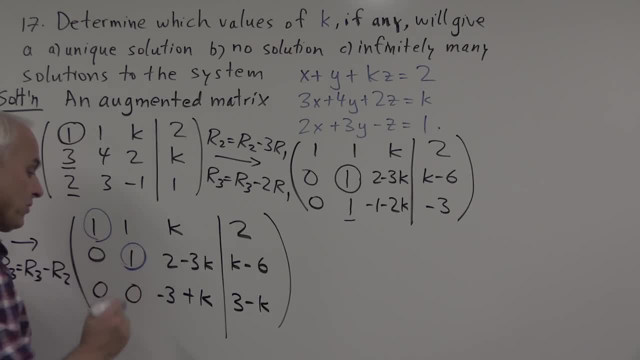 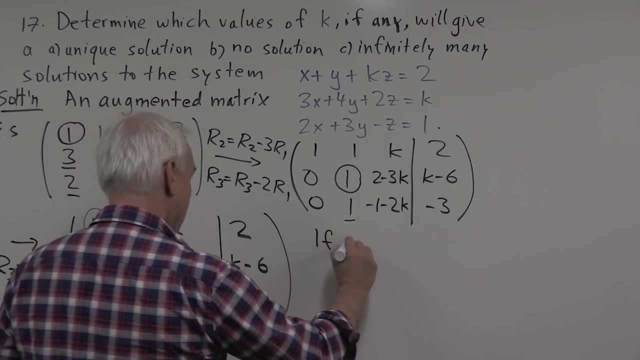 So here we have a leading entry, And here we have a leading entry And this is possibly a leading entry. It will be a leading entry if it is non-zero, So we can say that if minus 3 plus k does not equal 0,. 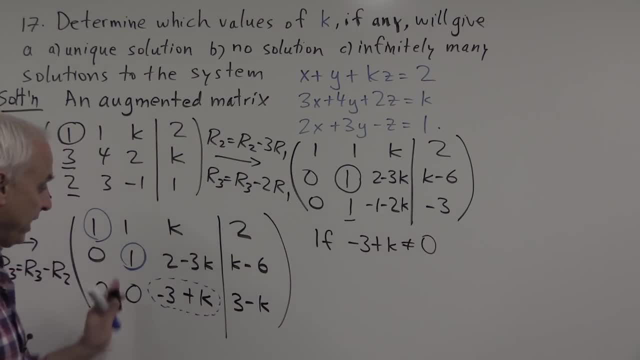 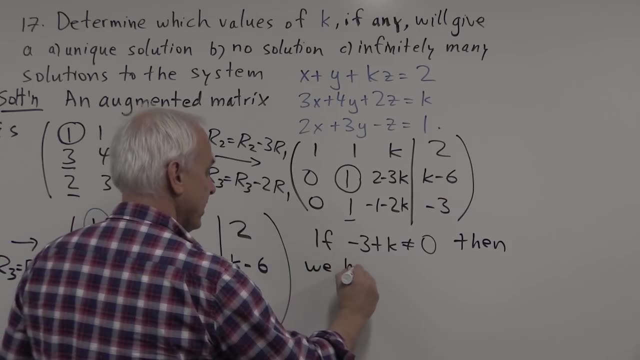 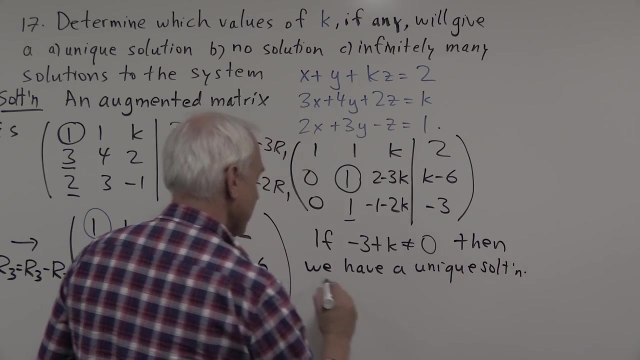 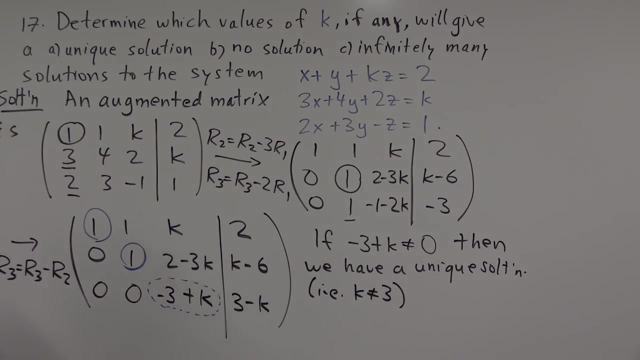 then this is a leading entry and we have three leading columns, Which means we have a unique solution. So, in other words, that's the case when k does not equal 3.. Suppose k equals 3.. In that case, this entry will be 0 and this entry will also be 0. 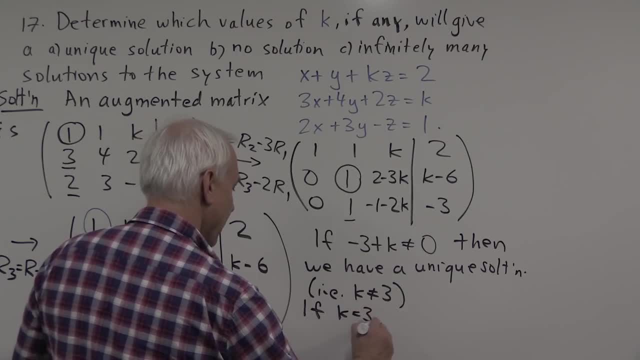 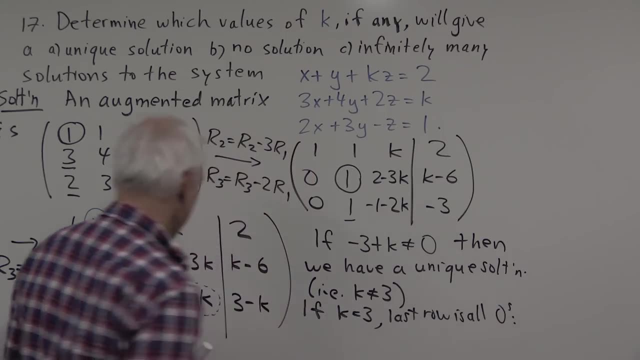 So if k equals 3, then the last row is all 0.. In which case, we will get a situation where we have two leading columns and one non-leading column, And then there is an infinite family of solutions, because we can set this variable to be a parameter. 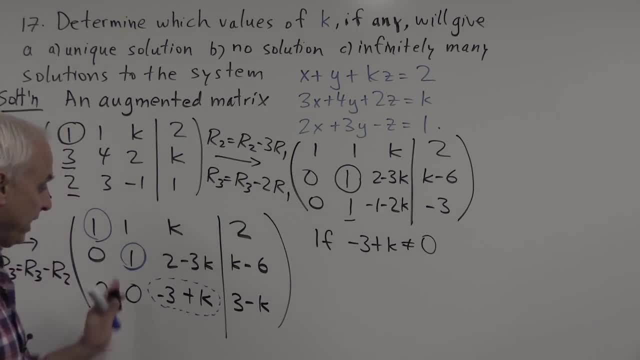 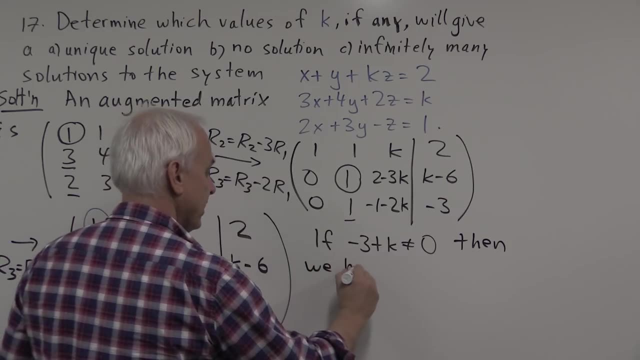 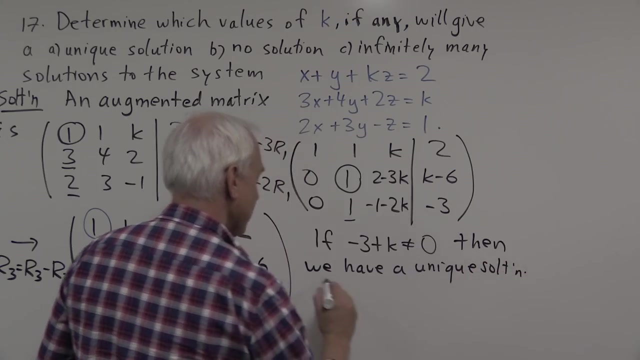 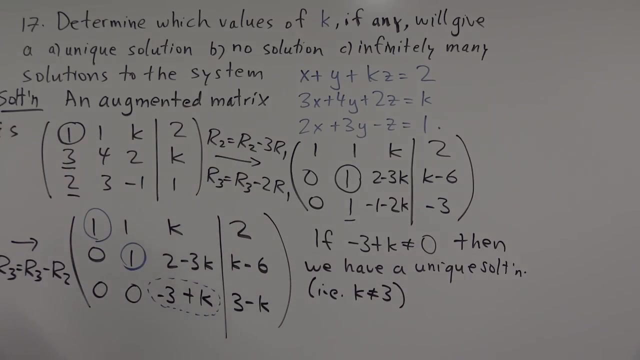 then this is a leading entry and we have three leading columns, which means we have a unique solution. So, in other words, that's the case when k does not equal 3.. Suppose k equals 3.. In that case, this entry will be 0, and this entry will also be 0.